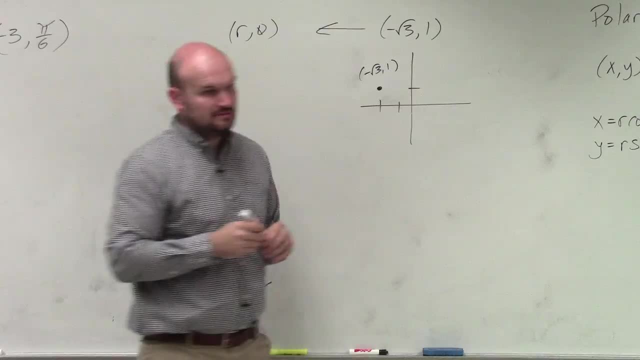 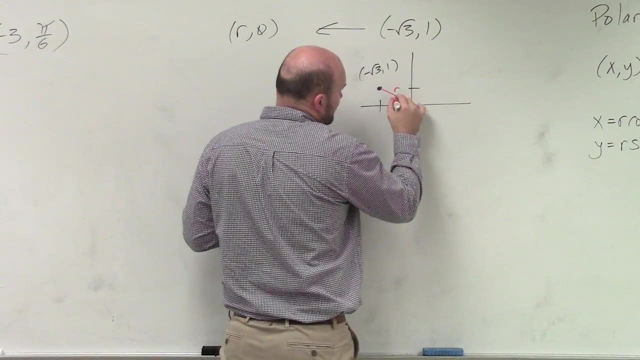 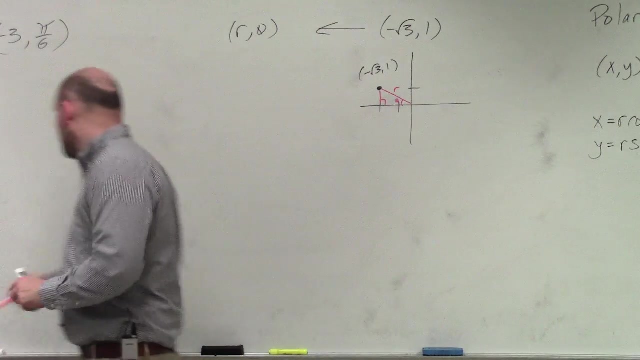 this point is, but I know it's somewhere in there- And again we're trying to write this in rectangular form, meaning we're trying to find this length r and this angle theta, So again create a triangle. We know this horizontal distance is negative square root. 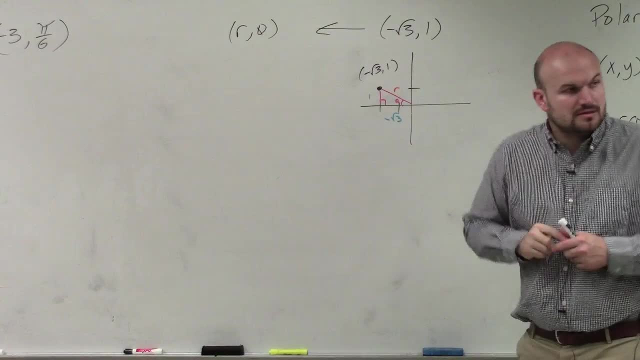 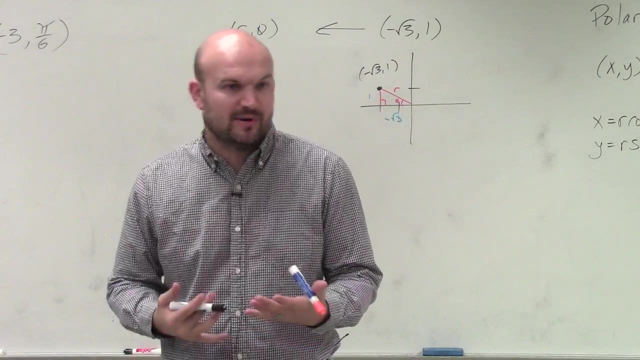 of 3, and we know the vertical distance is 1.. So do we have enough information to find r and do we have enough information to find theta? Bless you. Yes, There's no magic formula. you guys need to memorize. 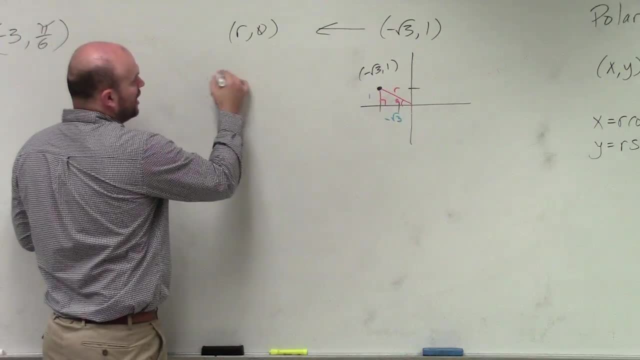 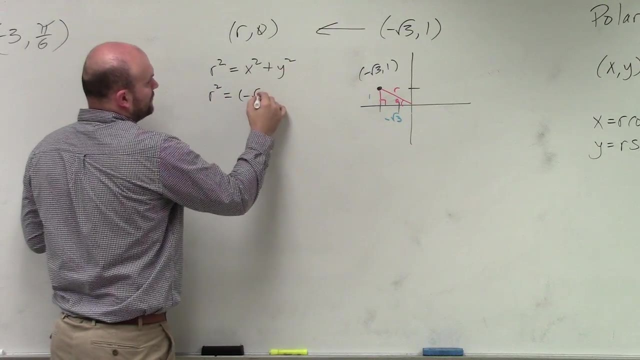 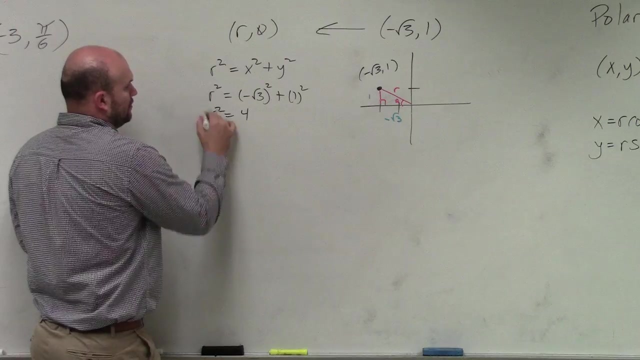 It's the same stuff we've been doing over and over. So to find r, r squared equals x squared plus y squared, r squared equals negative square root of 3 squared plus 1 squared, So that becomes: 3 plus 1 is 4.. 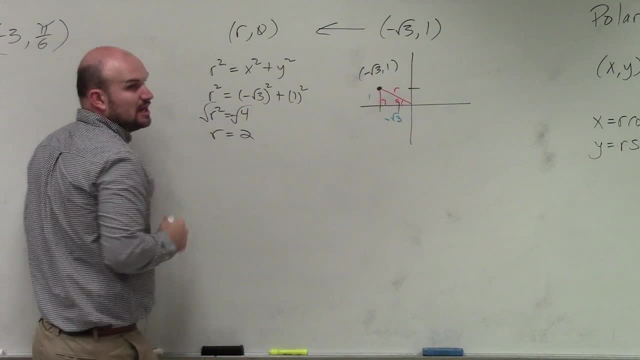 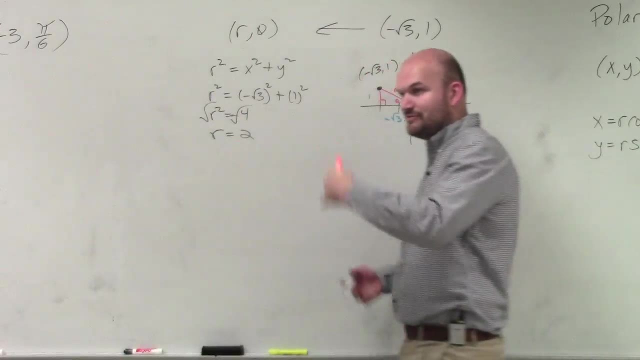 Root root r equals plus or minus 2, but since we're talking about distance, we're only going to deal with the positive 2.. However, if you remember what we talked about, that- positive or negative- you can do the inverse directional. 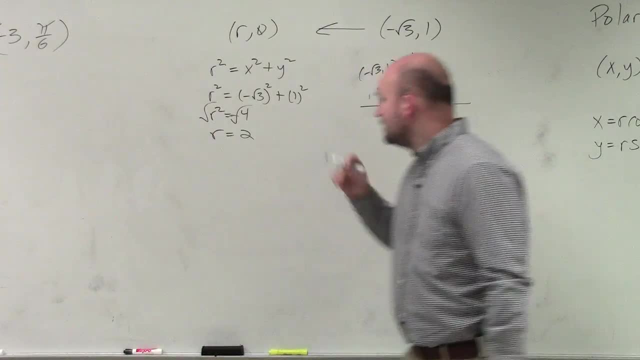 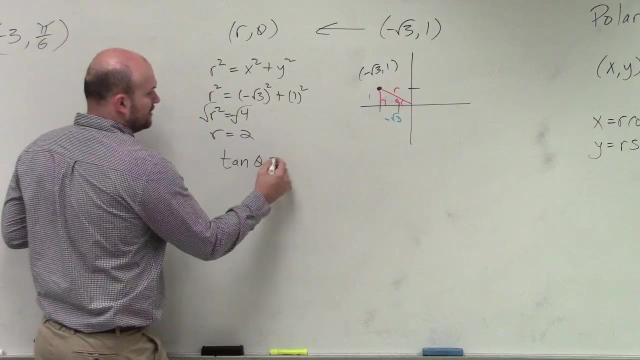 sign. So the negative can work. You just need to make sure you change your angle So there are r equals 2 in this case, And then we need to figure out the angle So you do: tangent of theta equals opposite over adjacent. 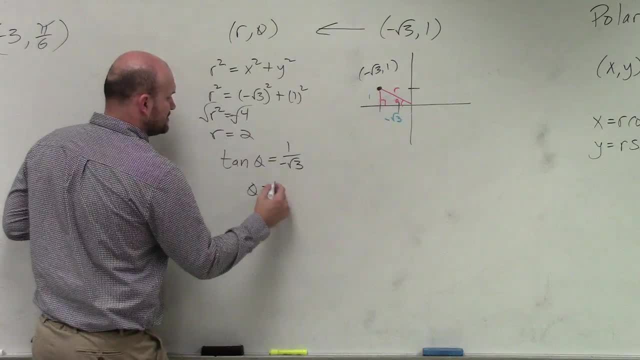 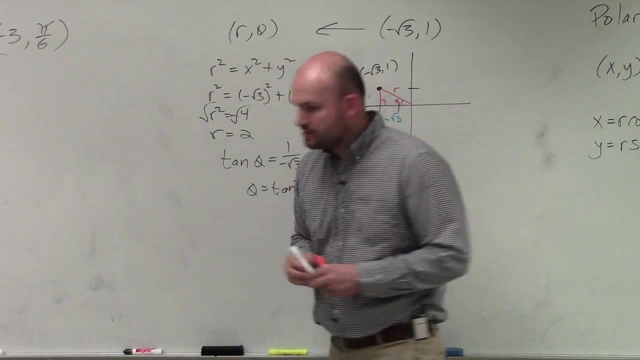 So 1 over negative square root of 3.. Therefore theta equals tangent inverse of theta. So you have 1 over negative square root of 3.. So when you go ahead and use a calculator, somebody stole my calculator. Here's my calculator. 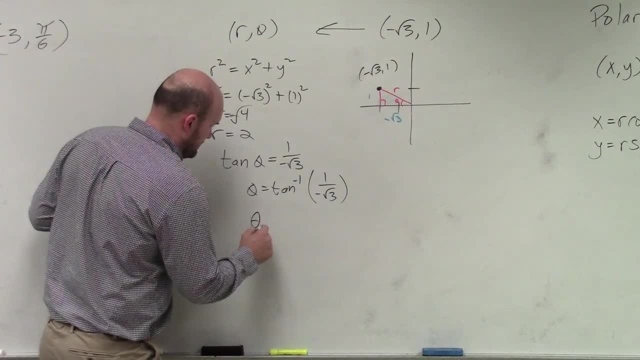 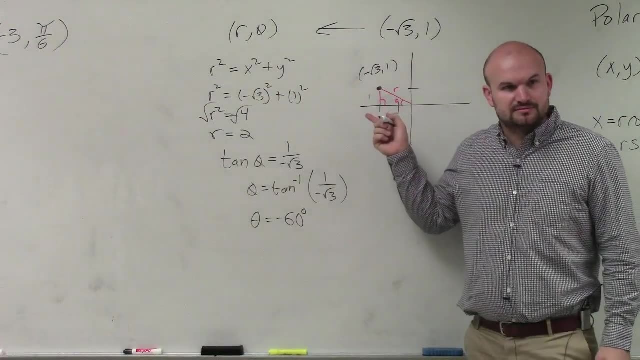 Negative 60 degrees. Now that is interesting Because I don't have a calculator, but it's just negative. Well, there's a problem. Does this angle look like negative 60 degrees? Are you sure it's negative 60 degrees? 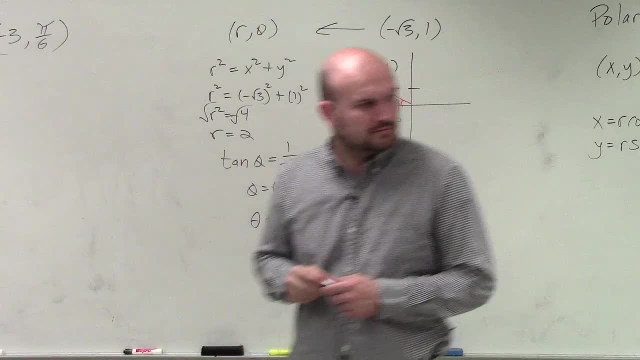 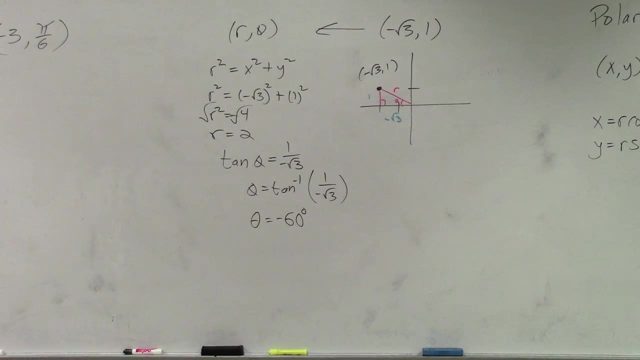 Negative 1.81?. That's what it said. Can I see your calculator? Can I use yours? I just want to type it in: You got 30 degrees. No, that's right. I think 30 degrees is right. 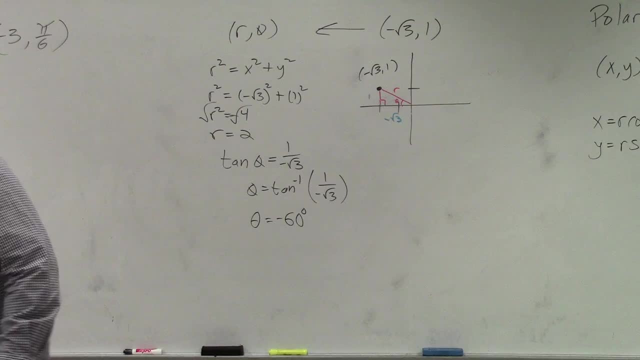 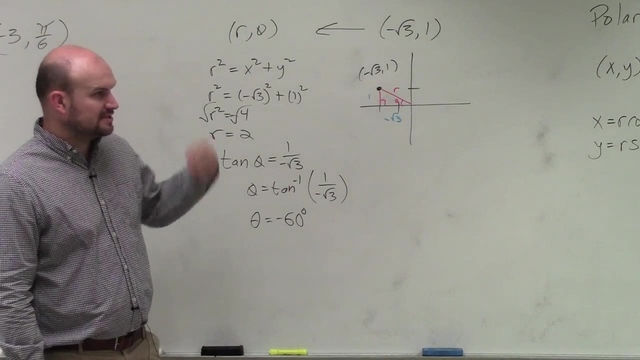 I don't know how you got 60 degrees. 30 degrees sounds right to me. It's going farther horizontally than it is vertically. Oh, you know what I did? I did negative square root of 3 over 1.. That'd be it.